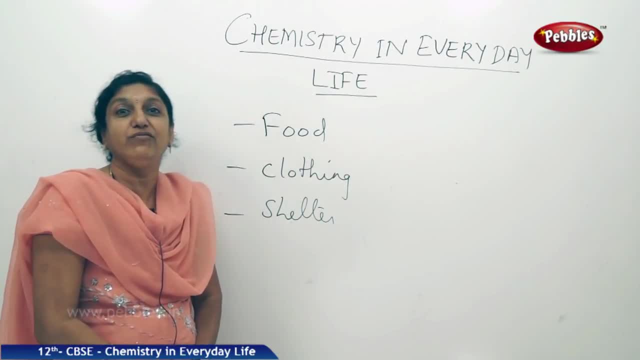 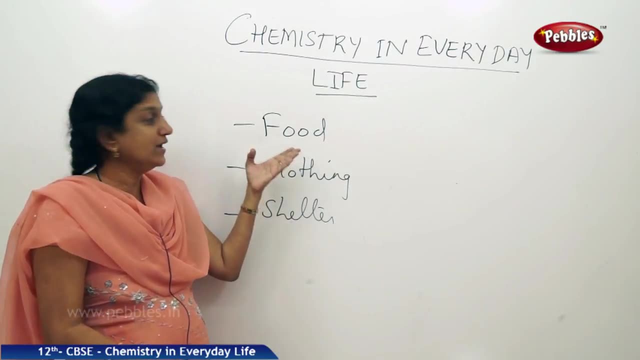 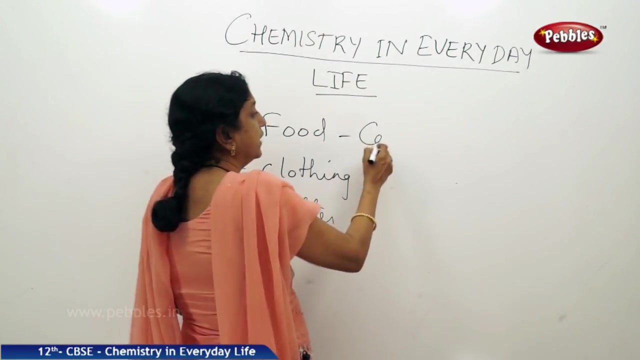 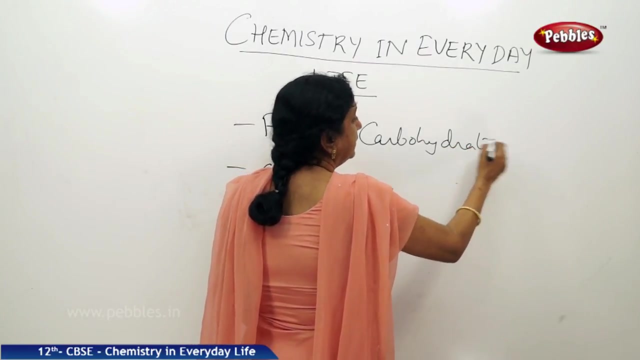 how they are undergoing chemical changes. It is due to that that life is being sustained here. So not only that. our basic requirements, we say, are food, clothing and shelter. Let us look at food. We say food can be divided into carbohydrates, proteins, lipids, carbohydrates. 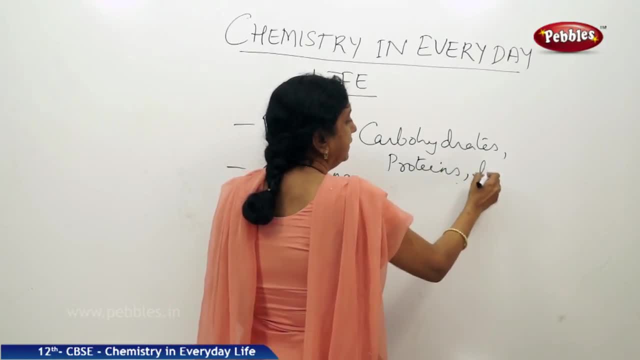 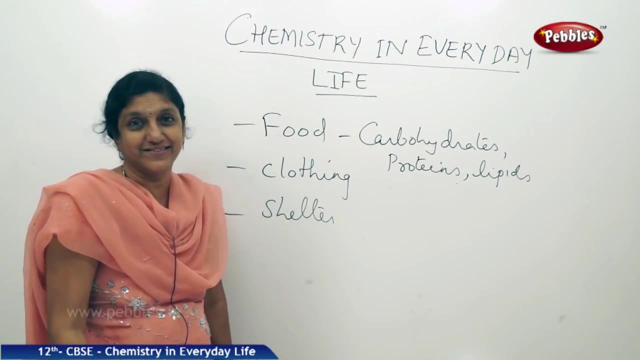 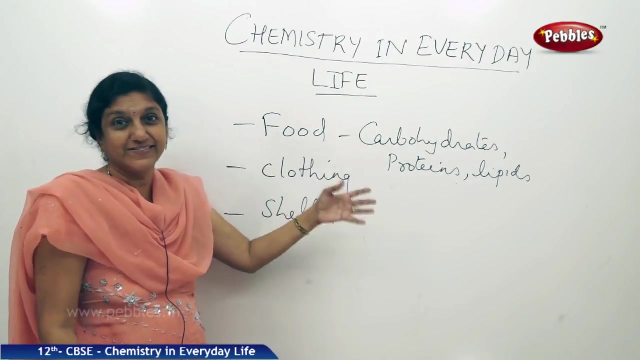 proteins, lipids, carbohydrates, proteins, lipids, carbohydrates, lipids, carbohydrates and so on. So whatever diet that you take for your existence or for sustaining life, all those materials are nothing but chemicals. So there is chemistry and chemical reactions involved. 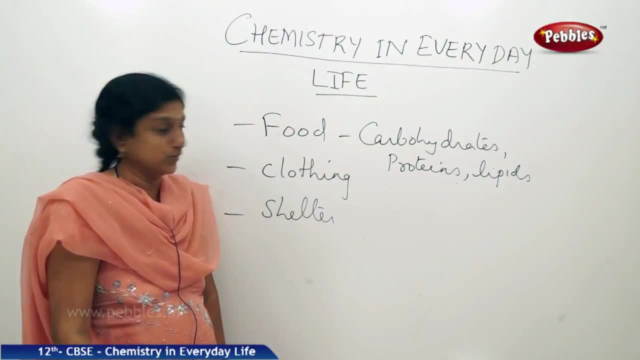 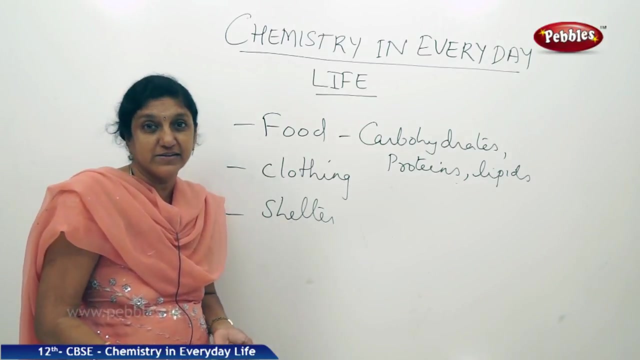 in the digestion of the food that you take in. also, And not only that clothing, you have natural fibers and you have synthetic fibers. They are all chemicals which are helping to clothe you. So all the clothes that we use for protecting and covering ourselves, they are also a collection of chemicals. 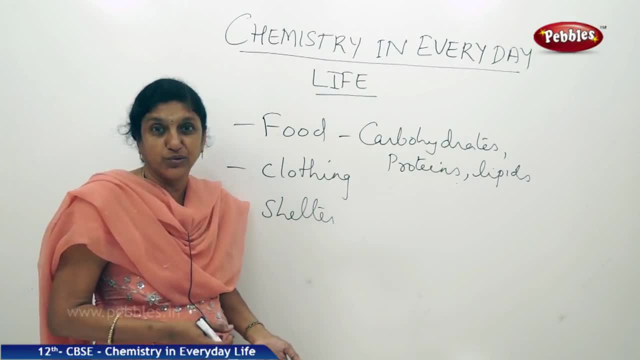 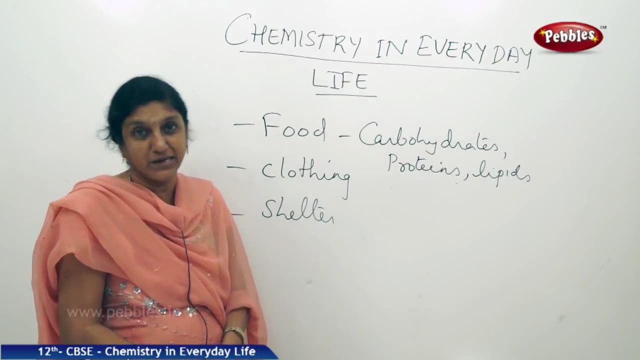 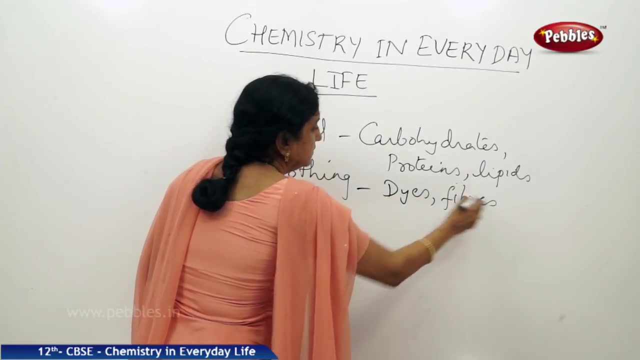 And not only that. you wear different colored clothes, So the dyes that are required to dye these clothes or color these clothes are also chemicals. And not only that, so the dyes and the fibers- these are what are required for clothing, isn't it? And they all involve. 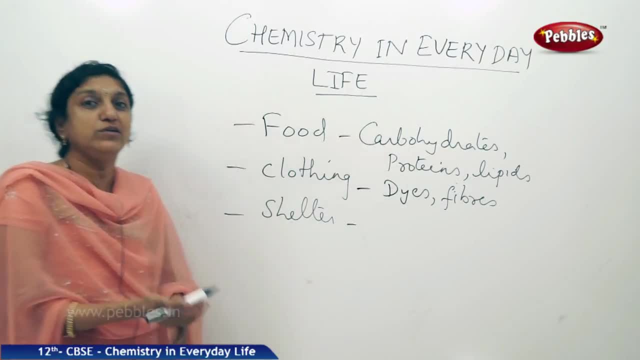 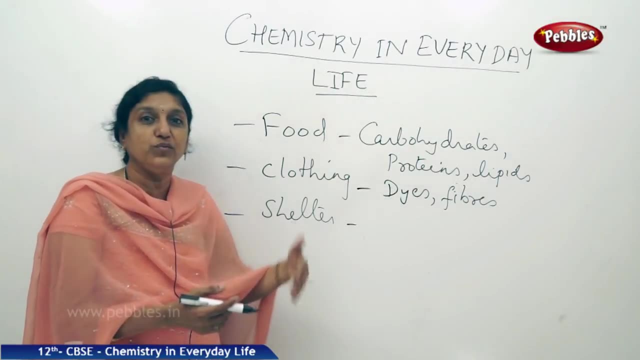 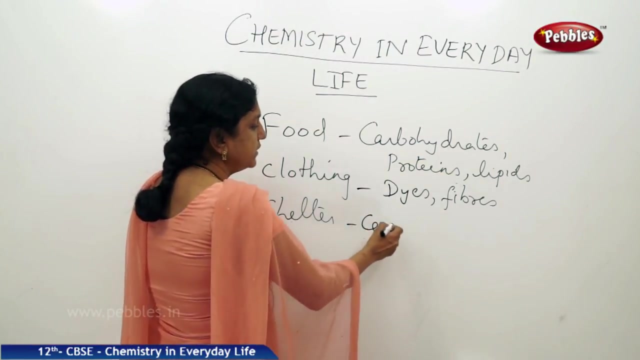 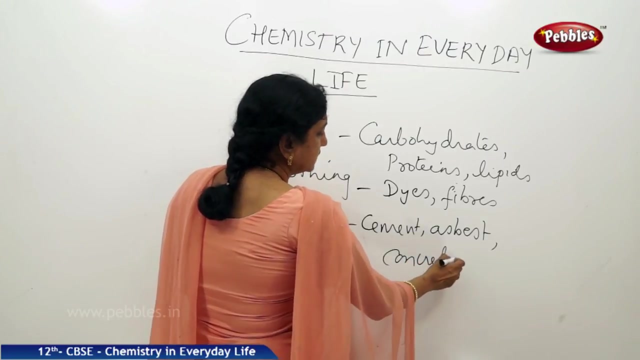 chemicals. Not only that: shelter. Now we need to live somewhere safe. So for that you construct different houses, And not only houses, various commercial establishments. So for all construction purposes you make use of what is cement, asbestos, you have concrete and so on, bricks. So all these materials are also chemicals. So you show me. 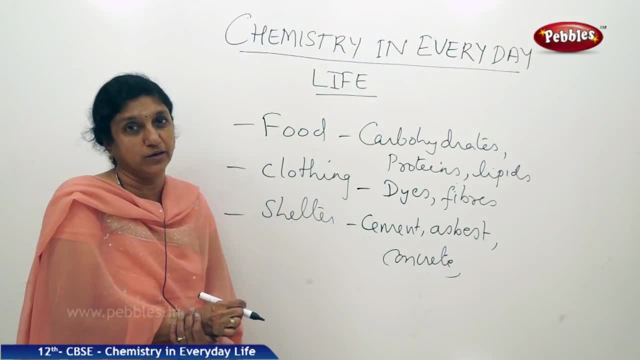 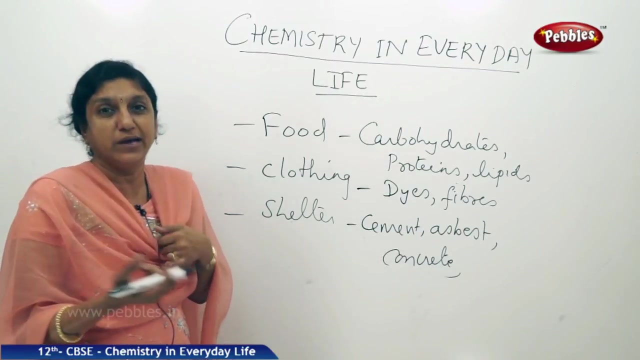 one walk of life where chemistry is not involved. So chemistry is involved in every sphere of life, Not only the basic requirements of mankind, even the very life itself. all living organisms are made up of biomolecules, which are nothing but chemicals. So 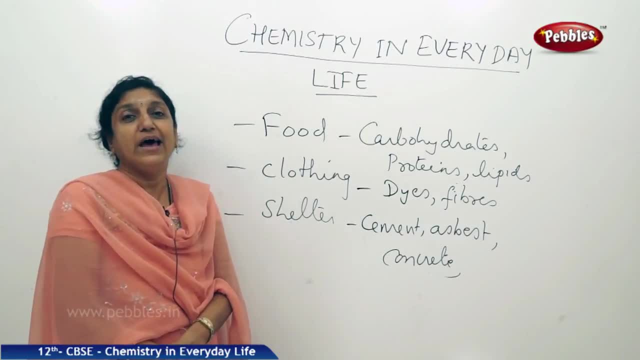 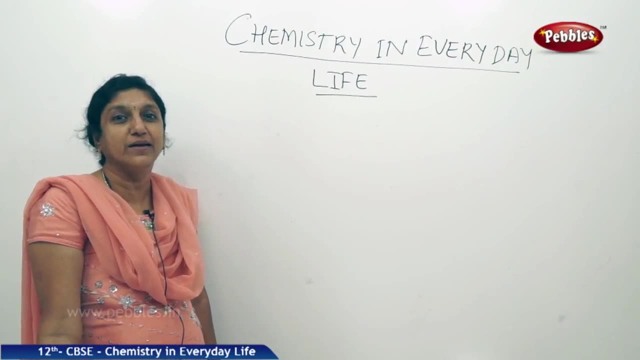 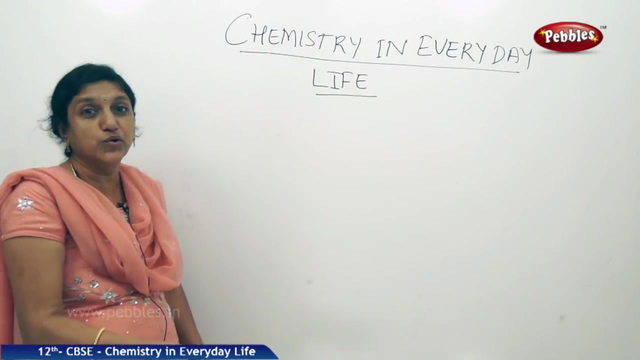 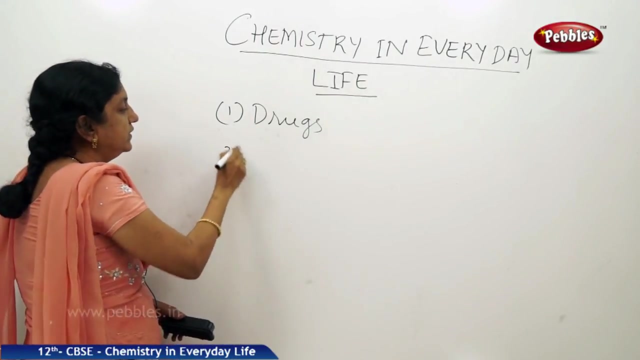 in this particular chapter, we will discuss the application of chemistry in three major areas. Now, in this discussion, we will examine three major areas in which chemistry plays a major role. So let us see what those major areas are. One is drugs, And the other that we will examine are: 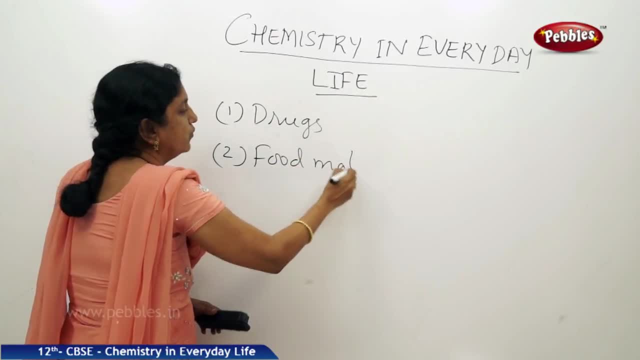 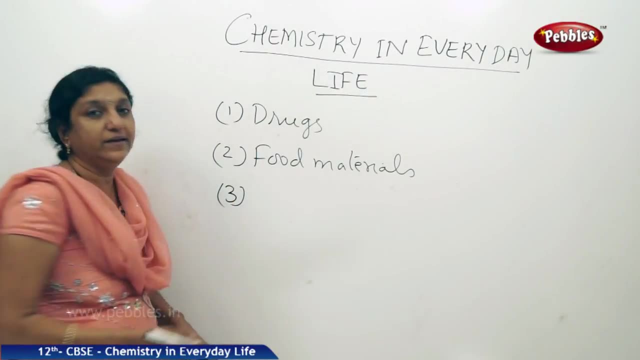 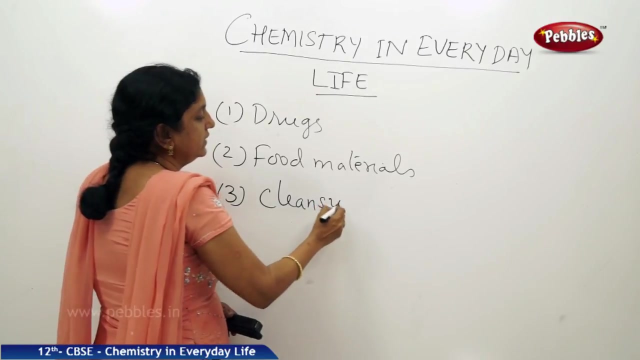 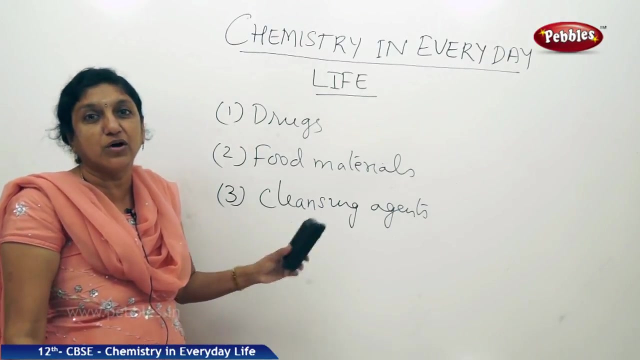 food materials. Now, what is the role of chemistry in these areas? Food materials. And thirdly, we will discuss about cleansing agents, Substances used for cleaning, Cleansing agents. So these are the three areas we are going to examine the action of chemistry or the role played. 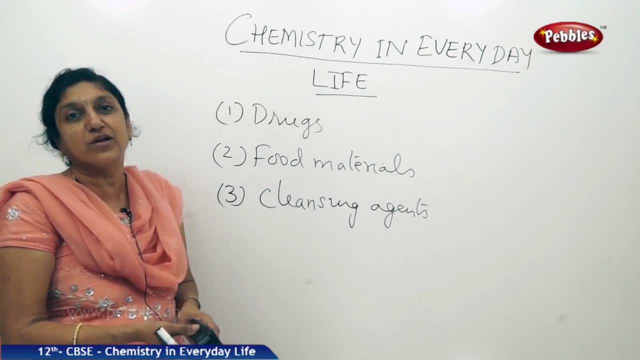 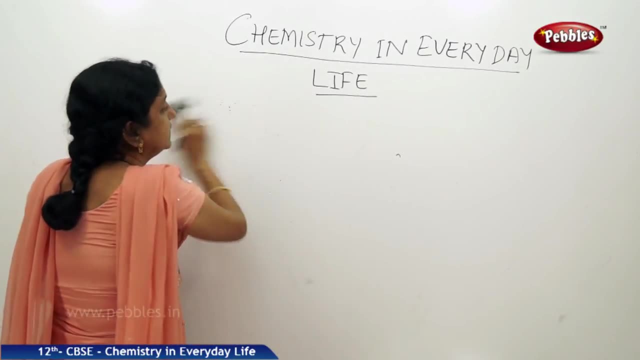 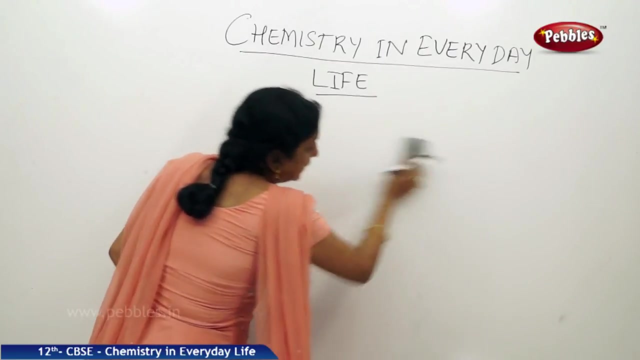 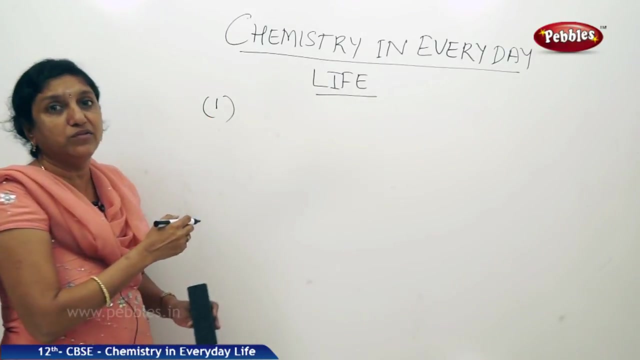 by chemistry. So let us begin our discussion with the application of chemistry in what are called as drugs, Right? So let us see what are drugs, how they are classified, how they act in the body and what biological response they produce in the body. So the first application of chemistry. 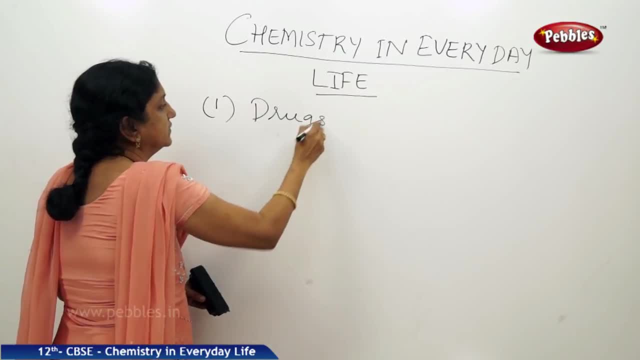 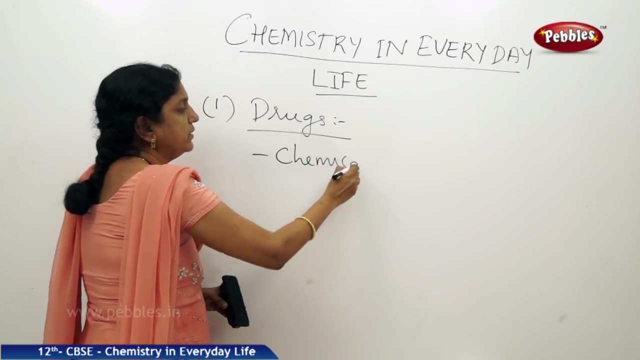 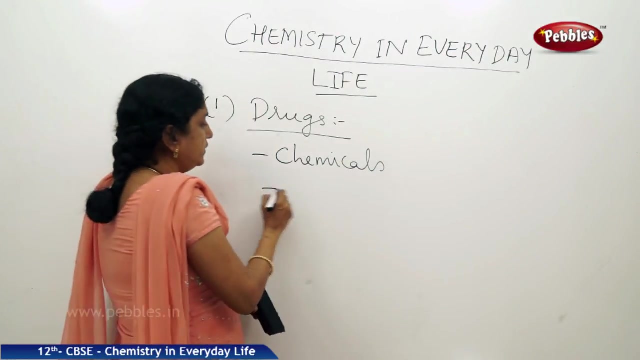 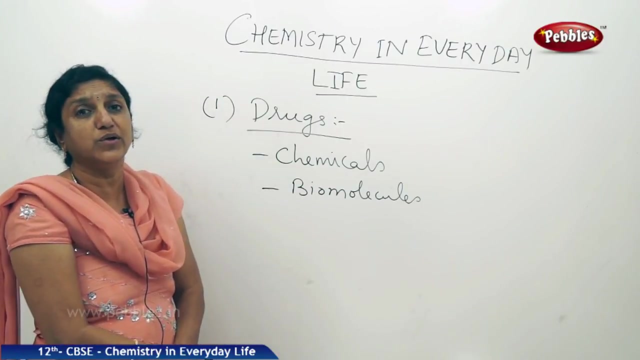 we shall study in what are called as drugs. Now, what are drugs? Drugs are nothing but chemical substances. They are chemicals, Right, and these chemicals, when taken, they interact with biomolecules in our body. We have studied about biomolecules, studied about biomolecules, so various biomolecules you have like proteins, carbohydrates, lipids. 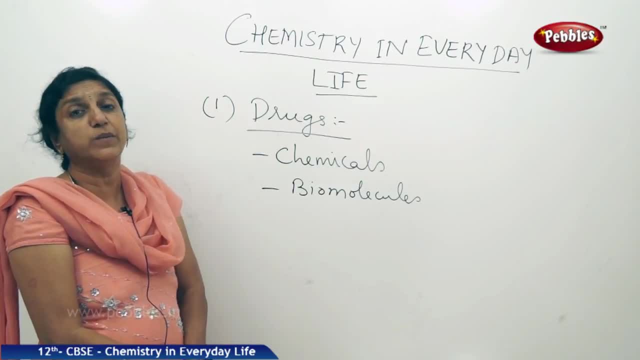 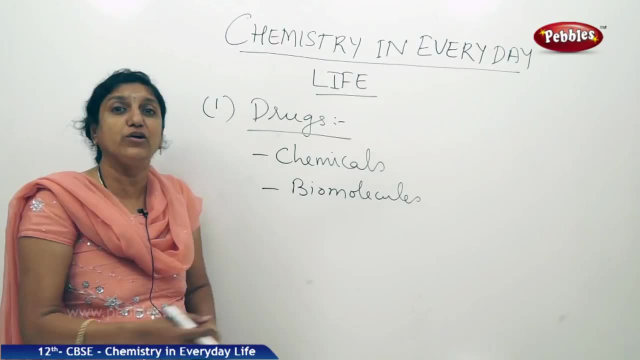 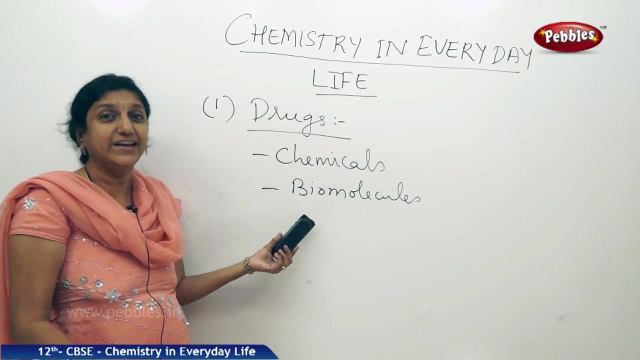 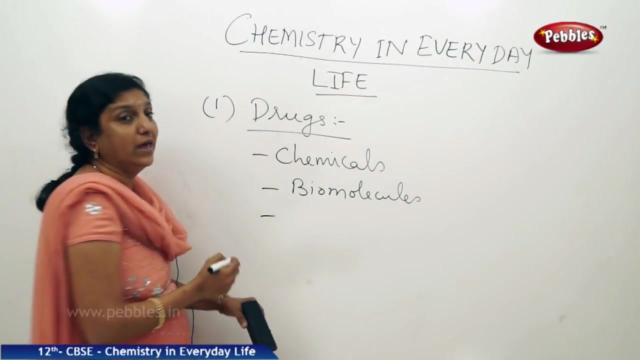 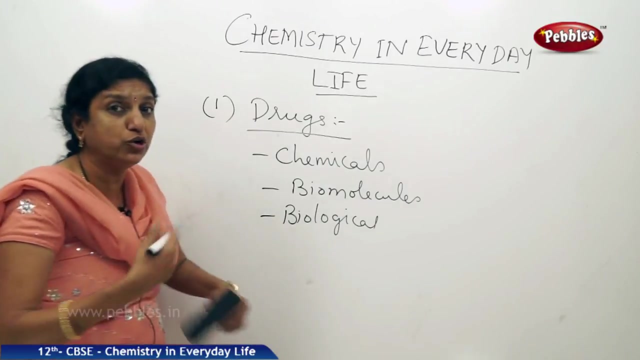 nucleic acids and so on. so there are various biomolecules which are playing a coordinated role inside the body for the smooth running of that particular organism. so drugs are nothing but chemicals which directly interact with biomolecules inside living systems and they produce a biological response. biological response in that particular organism. they produce a. 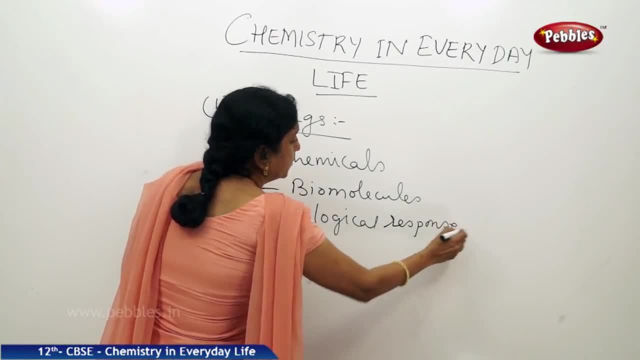 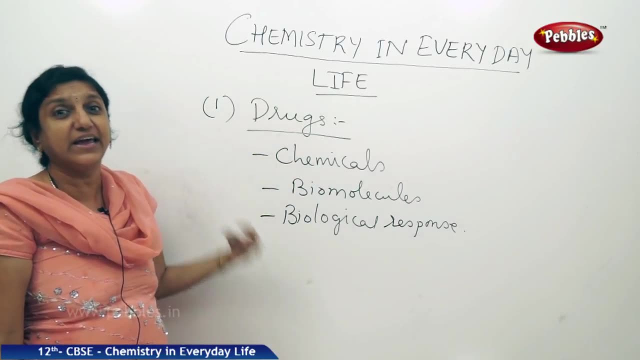 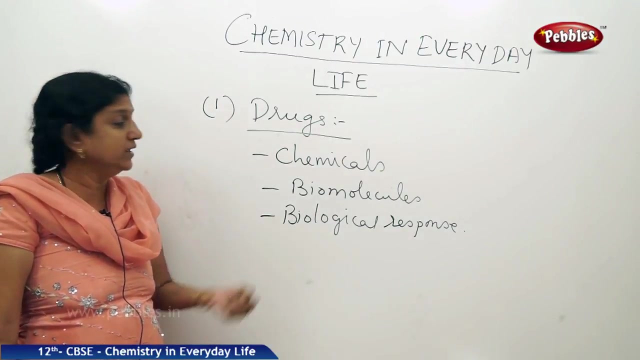 response, which is called as biological response. so how do you define drugs? drugs are defined as the chemicals that are taken and, after being taken, they areаться make them manageRight, They interact with the biomolecules present in the living system and they produce a biological response. 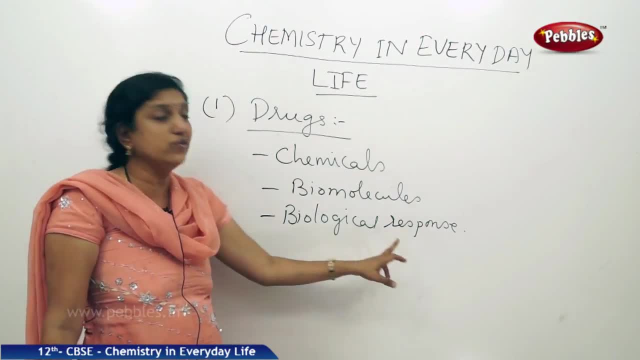 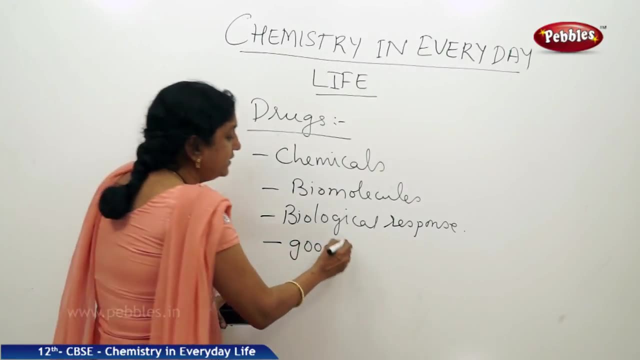 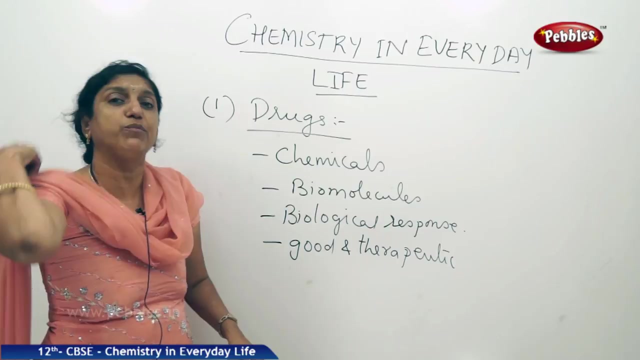 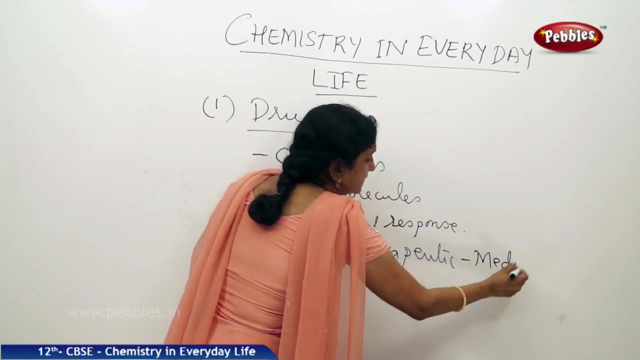 Such chemicals are called as drugs. Now, this biological response, if it is good or favorable for the organism and it is therapeutic, that means it solves certain problem that is there in the body, Then you call such drugs as medicines. So there is a slight difference between the words drug and medicine. 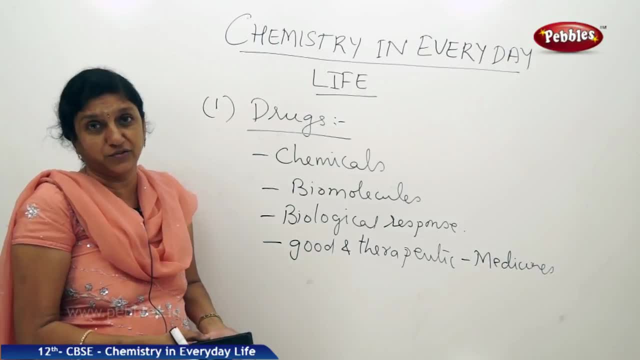 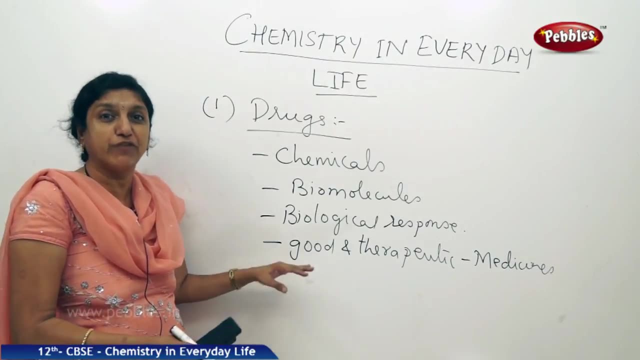 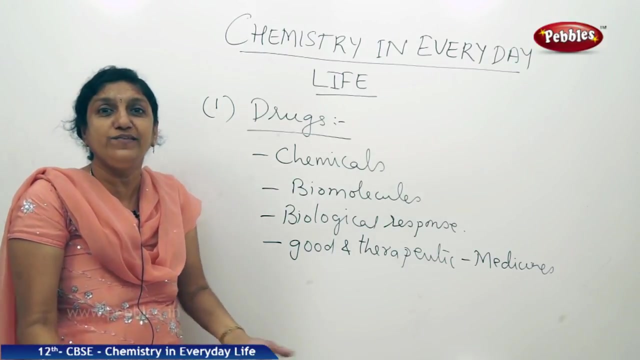 So drug is any chemical which produces a biological response when it interacts with the biomolecule of the living system. If that response is good, favorable and therapeutic, then you call that particular drug as a medicine. That is, when you fall sick, you take medicines, isn't it? 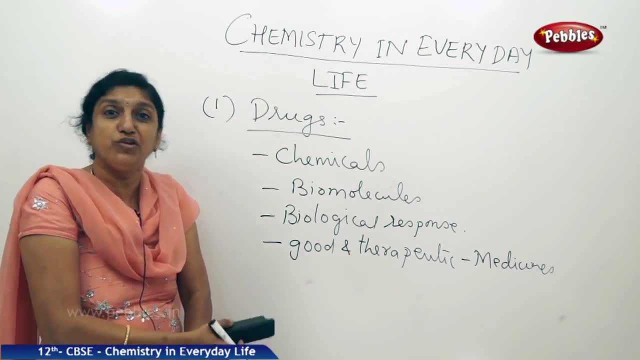 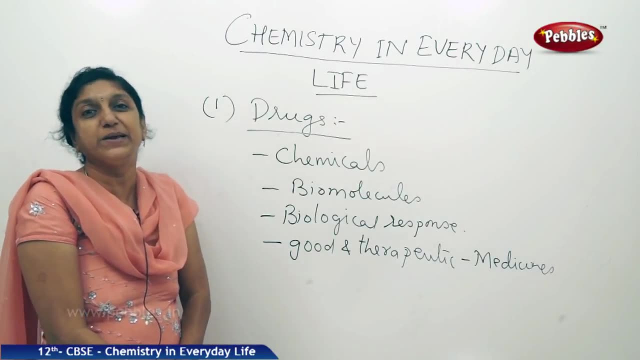 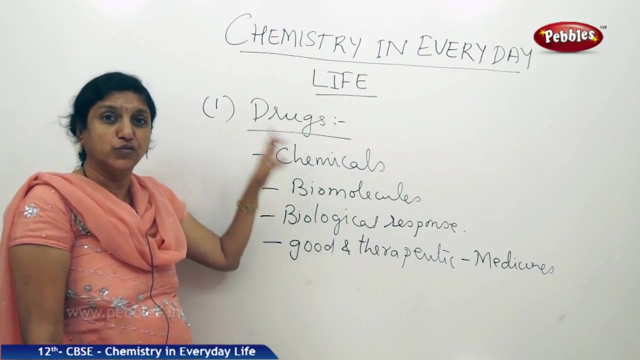 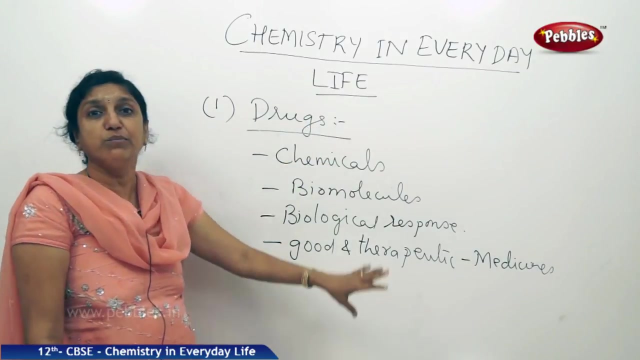 So medicines are good. So medicines are nothing but drugs or chemicals which produce a favorable biological response in you, not only you, any organism which is being treated, right? So this is the distinction between a drug and a medicine. So, whether it is drug or medicine, both of them are chemicals, right, but both of them. produce a biological response. If the biological response is good and therapeutic, Then you call that particular drug as a medicine, right? So after having defined what is a medicine, Let us go further and see what are the various types of drugs that are available. How do you classify these drugs? right Now, these drugs are usually low molecular mass substances. how low? hundred to five hundred unified. So the molecular mass of drugs usually lies in the range they are considered as low molecular mass chemicals. So it is between hundred and five hundred unified mass units, right? 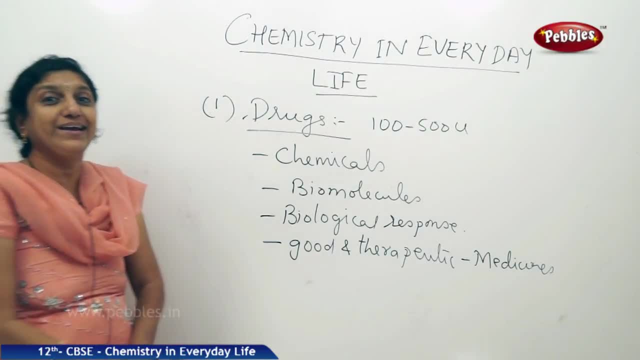 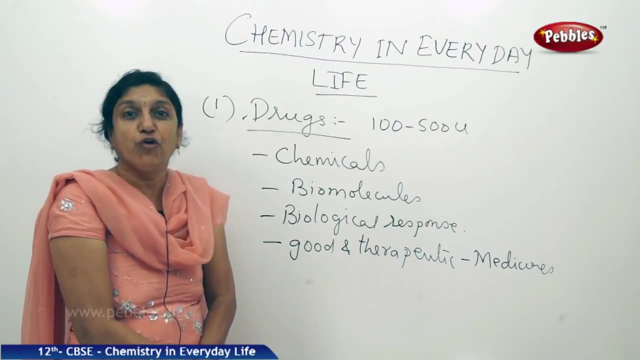 And these drugs if they are used for creating a therapeutic activity, then that process of using drugs for therapeutic action that is called as therapeutic activity. So this is the process of using drugs for therapeutic activity. So this is the process of using drugs for therapeutic activity. 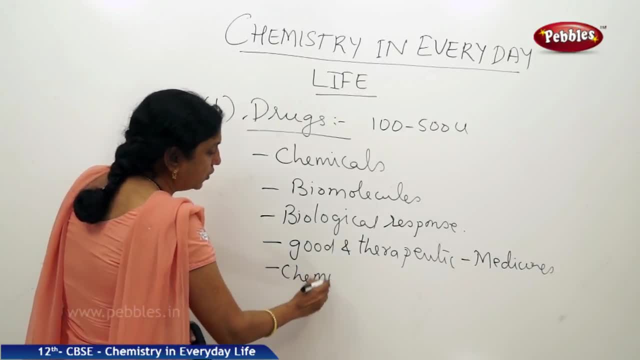 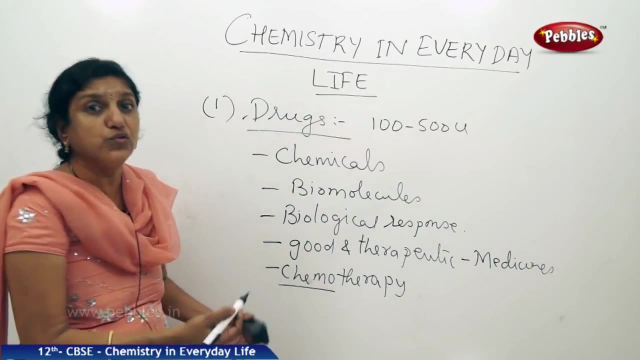 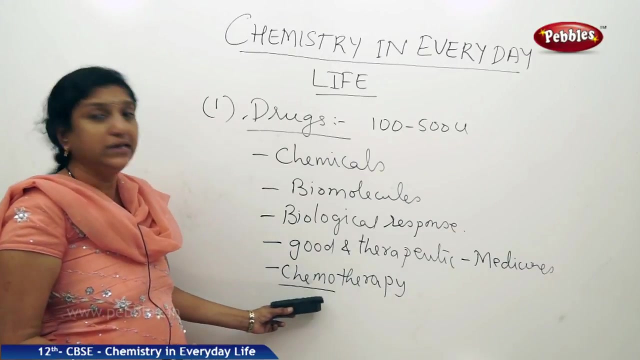 Now let us what is chemo- Chemotherapy. So let us understand the meaning of this word: chemo therapy. So what is chemo? Chemo means use of chemicals, So that is reflected by this first part of the name. that is chemo. 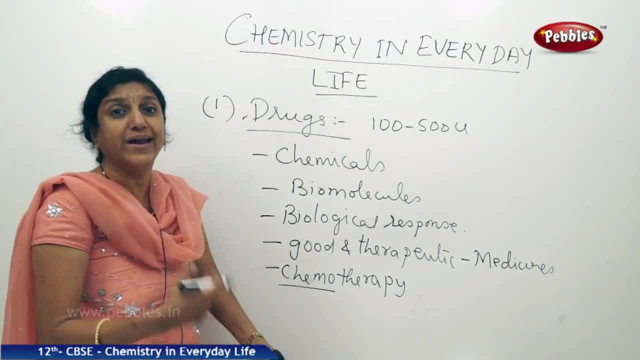 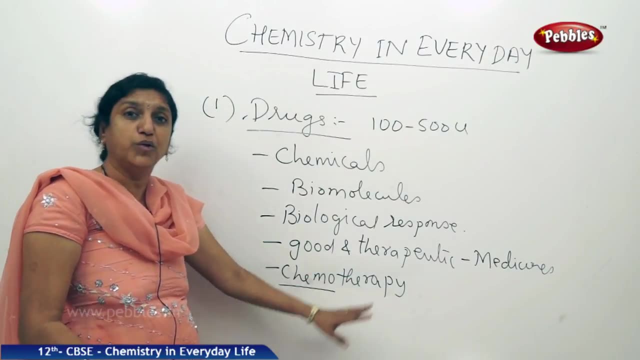 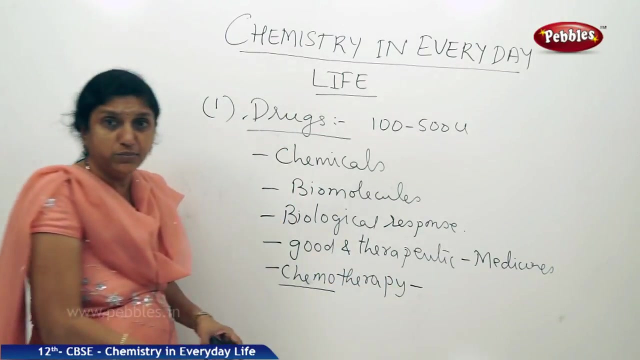 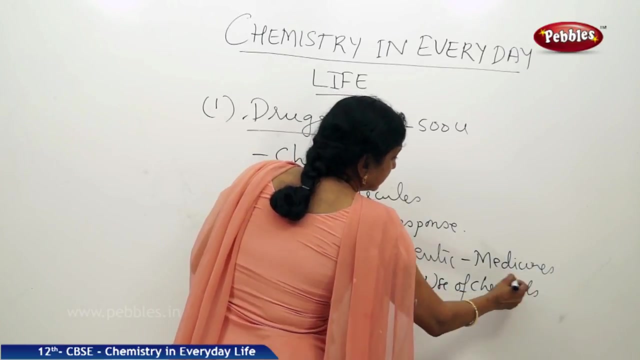 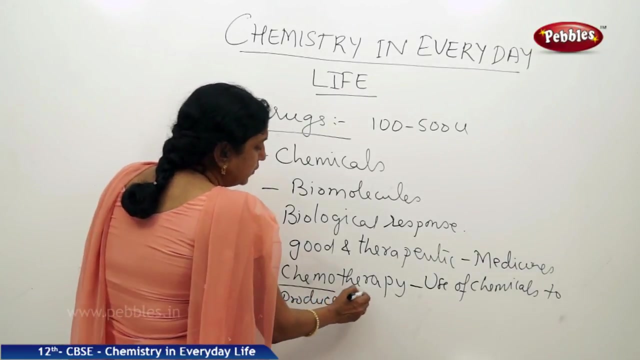 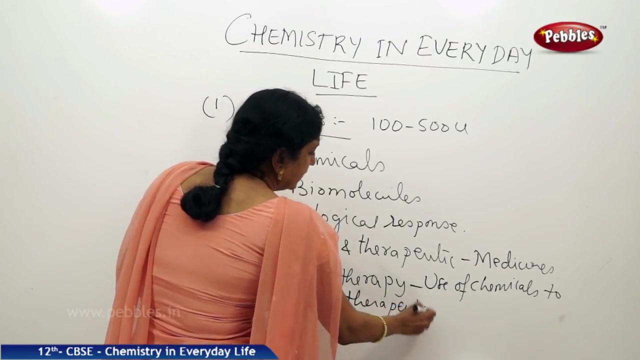 And therapy means therapeutic response or activity. If these chemicals are able to produce, then that process of using chemicals for producing therapeutic activity that is called as chemotherapy. So how do you define chemotherapy? It is use of chemicals to produce therapeutic activity. that means for treatment, therapeutic. 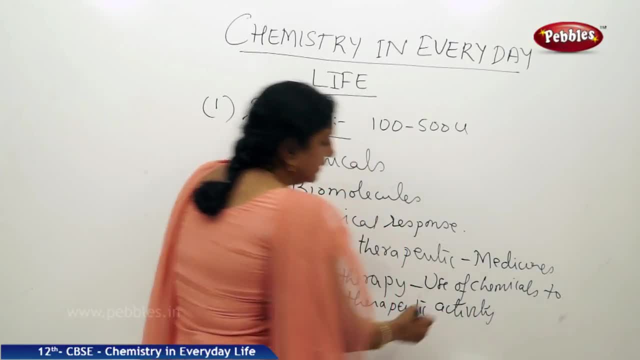 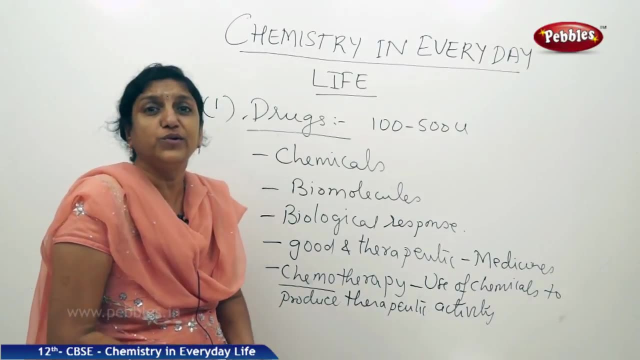 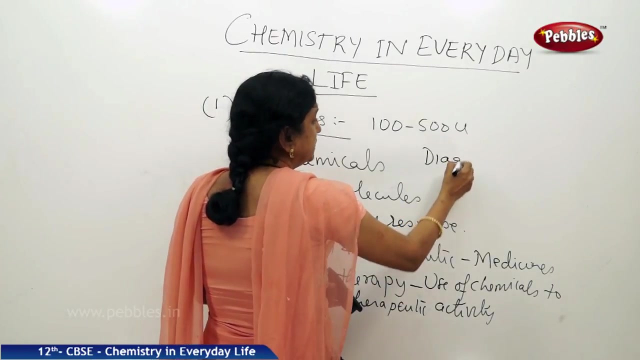 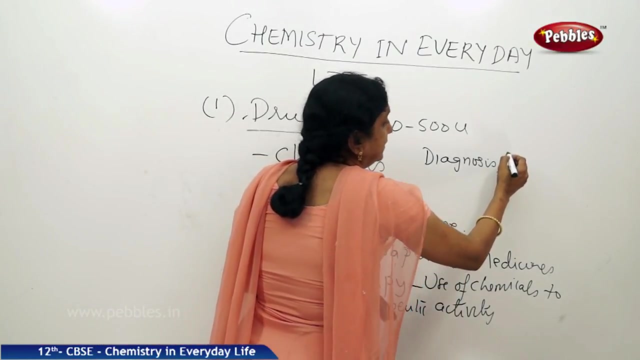 activity. Why do we use medicines? Medicines are used to diagnose, to prevent and also to treat diseases. So drugs or medicines are used for these purposes. What is that? Diagnosis? that means you find out what the problem is. that is diagnosis. Then you have treatment: how to treat, solve that problem. 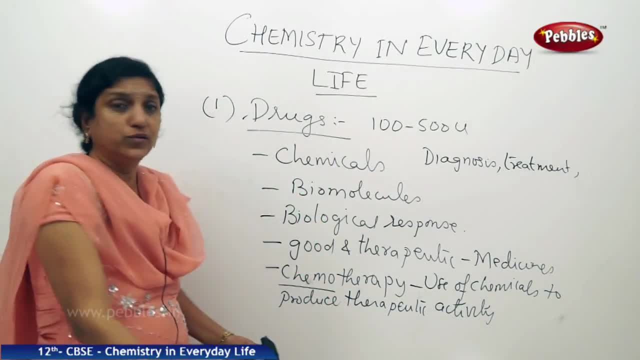 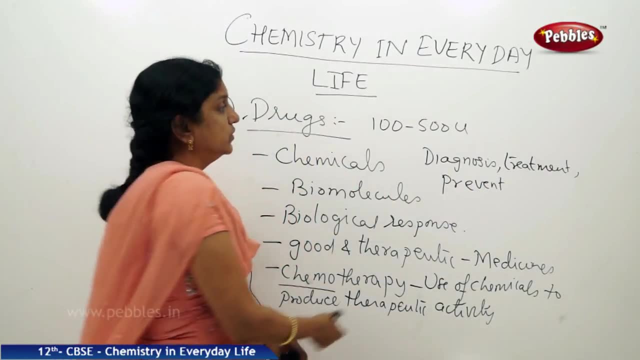 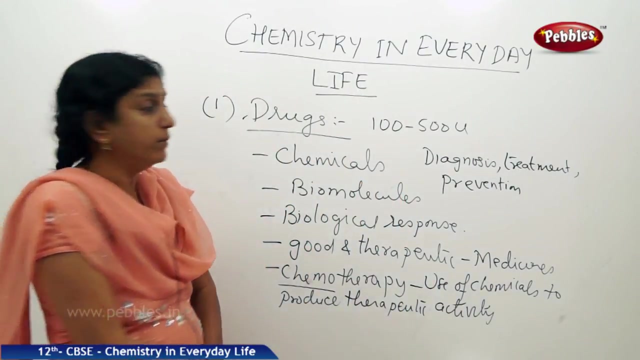 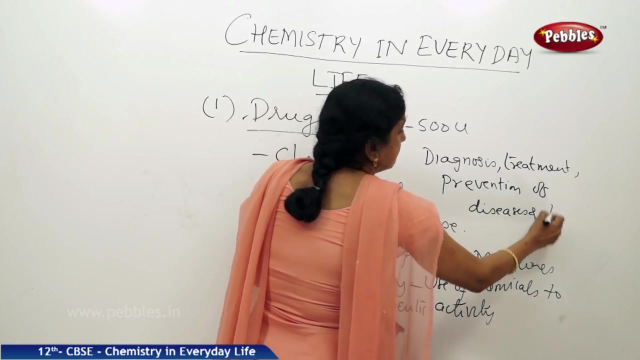 there treatment And also for prevention. So you have these vaccines which are used to prevent various types of diseases. So diagnosis, treatment and prevention are the main key roles played by medicines for prevention of diseases and disorders. So let us sum up: what are drugs? 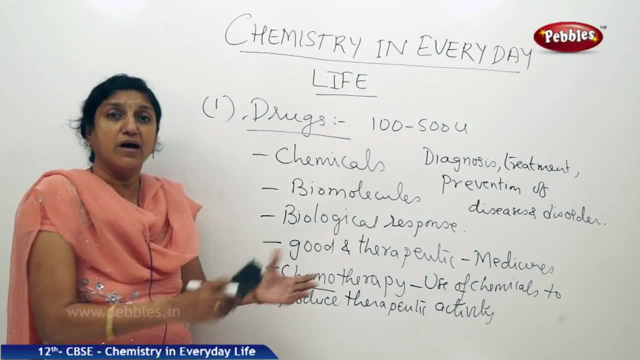 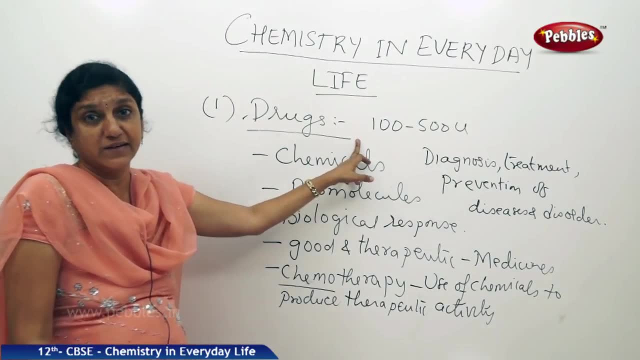 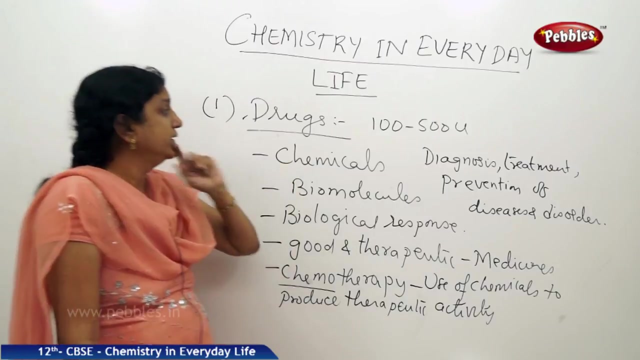 What is the role they play and why we require them, and how you differentiate between a drug and medicine. As we said, drugs are low molecular mass chemicals which have their molecular mass in the range 100 to 500 U. They are basically chemicals. They interact with biomolecules in living. 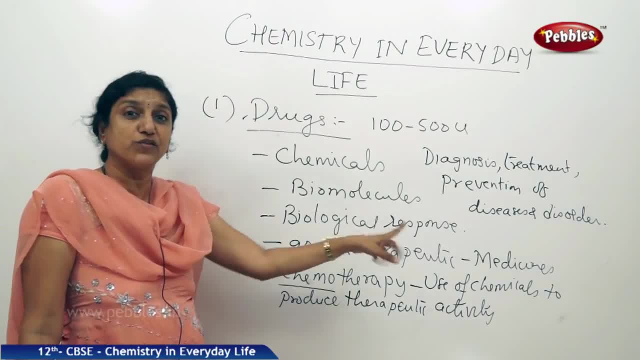 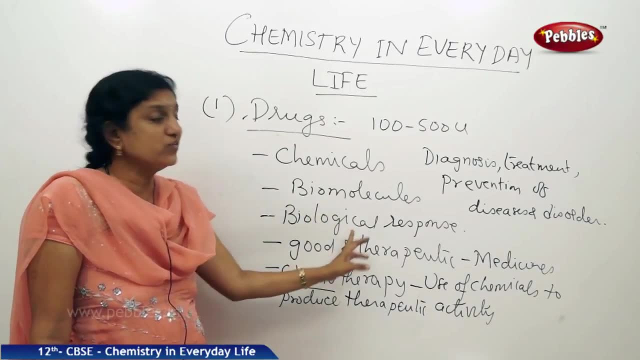 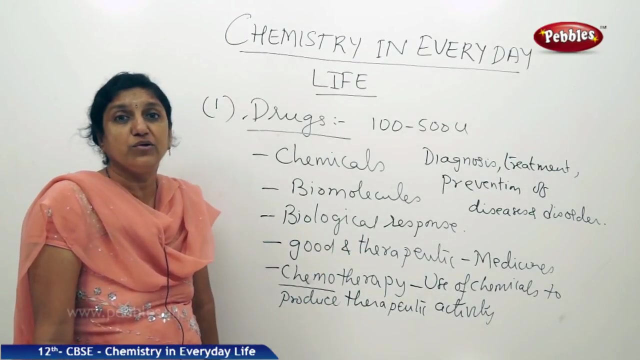 systems and they produce a biological response. due to interaction of these drugs with biomolecules in living systems, Biological response is produced. If that response is good and therapeutic, then you say those drugs are called as medicines. And why do we use medicines For the purpose? 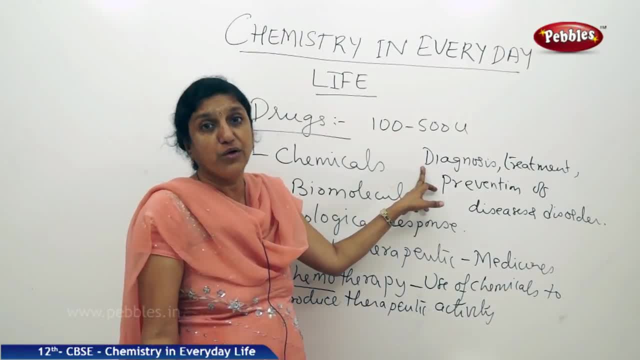 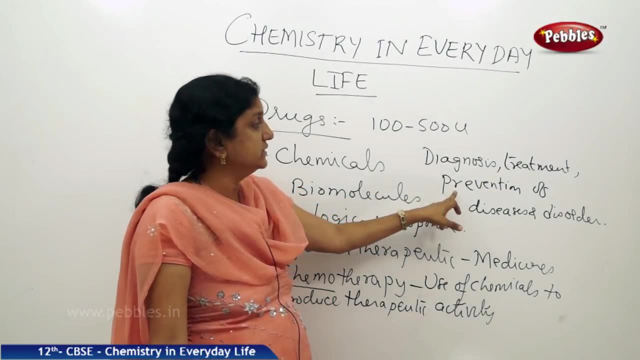 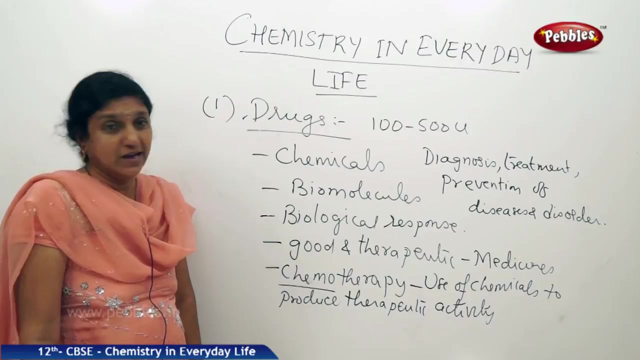 of diagnosis, That is, to find out what is wrong with that particular person or organism, To treat Certain diseases, whatever disease it is, and for the prevention of diseases and disorders. Prevention usually involves the usage of vaccines. Then we define the word chemotherapy. So from 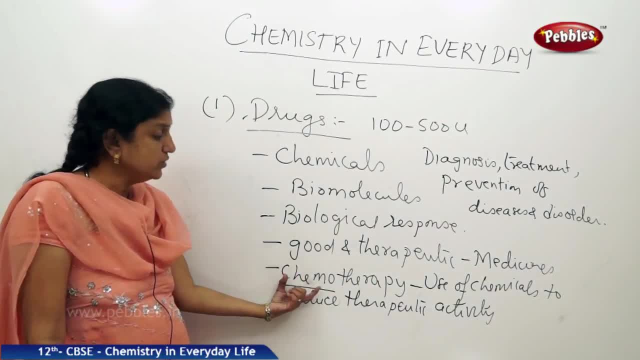 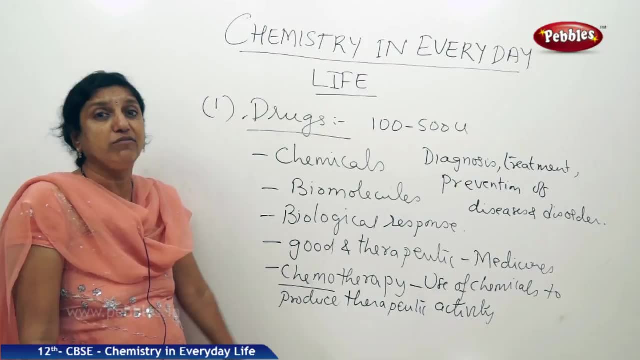 the name itself you can guess: chemotherapy is the use of chemicals for producing a therapeutic activity. So the treatment that you are giving with the help of chemicals, that is called as chemotherapy. What is chemotherapy? Now let us go on to how these various drugs are classified. So drugs are usually classified. based on four important aspects.